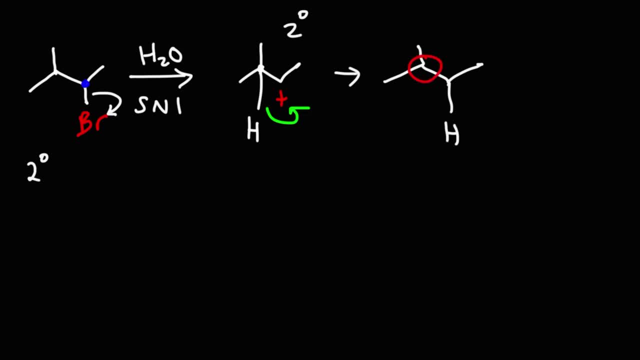 And here is that hydrogen now. Now this carbon lost a bond, so it's going to carry a positive charge. So now we have a tertiary carbocation as opposed to a secondary carbocation, And the reason why this rearrangement occurs is due to an increase in stability. 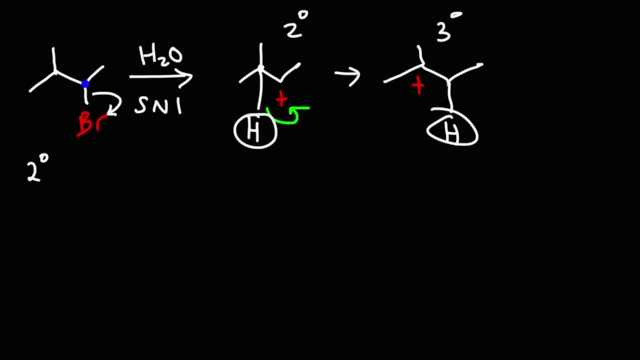 By moving the hydrogen from this position to that position, the carbocation becomes more stable. So it's going to do that. It wants to adopt the most stable configuration possible that it can find. So that's the driving force for a rearrangement reaction. 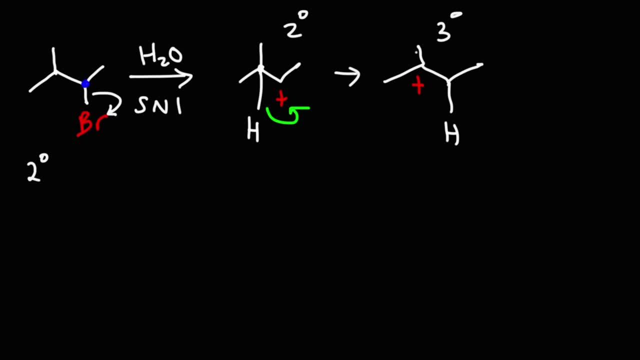 It's stability. So, now that we have this tertiary carbocation, what's going to happen? Once we form this carbocation? it's going to react with the solvent. When the solvent behaves as a nucleophile, what you have is a sylvalesis reaction. 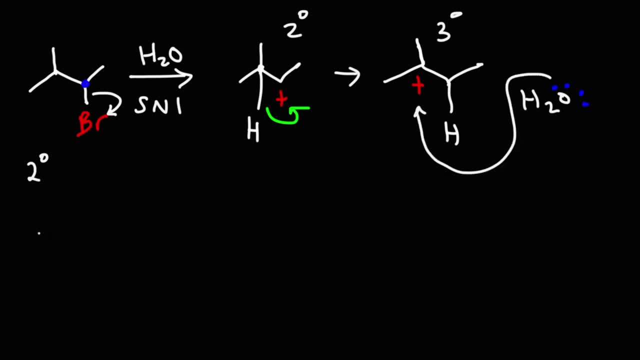 The nucleophile is going to combine with the carbocation, giving us an oxonium ion Which looks like this. Now, in the next step, another water molecule is going to come to remove a proton, And the end result is that we're going to get a tertiary alcohol. 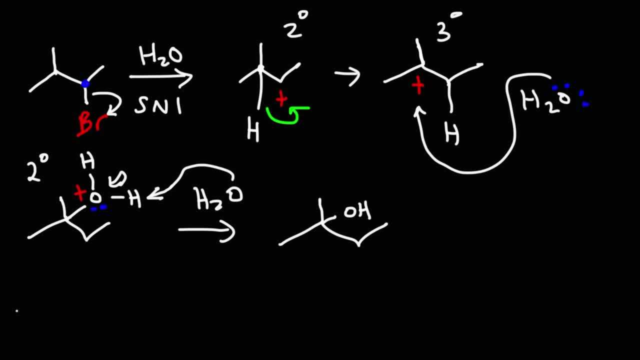 Particularly 2-methyl-2-butanol. So we're going to get a tertiary alcohol. So that's going to be the major product for this particular example. So make sure you understand this: If you have a secondary carbocation next to a tertiary carbon, you're going to get a hydride shift. 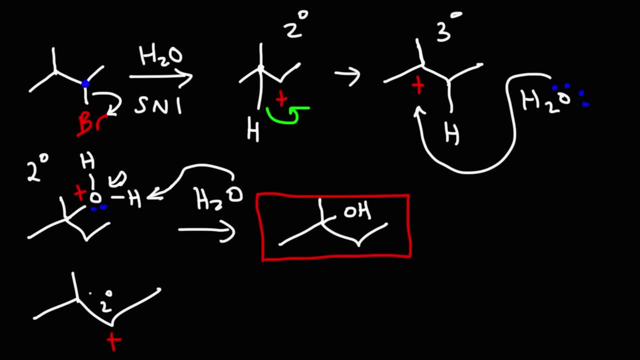 Now let's say, instead of a hydrogen, that we had a methyl group. This will be a quaternary carbon, So we're going to get a tertiary carbon. In this case, we can get a tertiary carbon, So we're going to get a tertiary carbon. 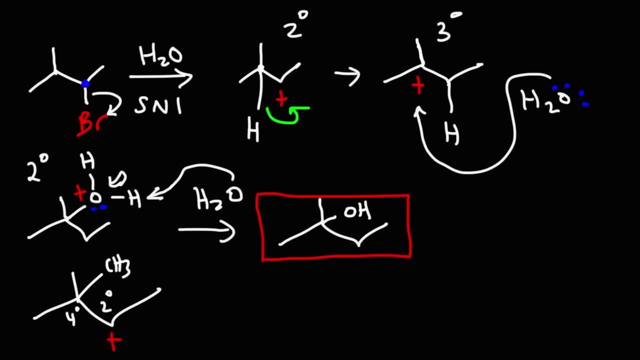 So we're going to get a tertiary carbon. So we're going to get a tertiary carbon. We can't get a hydride shift from that quaternary carbon, But what we can get is a methyl shift. So that's when they occur. Whenever you have a secondary carbocation next to a quaternary carbon, you're going to get a methyl shift. Or if you have a primary carbocation next to a quaternary carbon, that too can create a methyl shift as well. Now let's try another example. 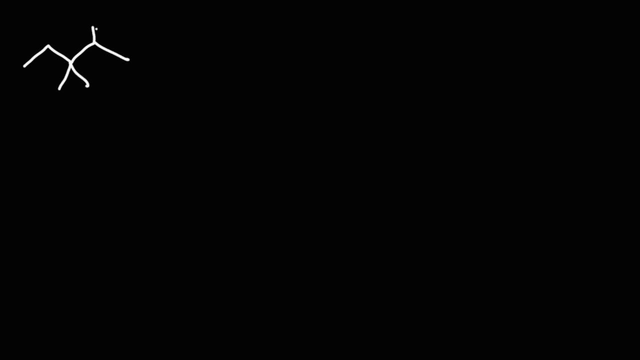 So here we have 2-bromo-3,3-dimethyl-pentane. This time we're going to react it with methanol as opposed to water, So feel free to pause the video and try this example. Determine the major mechanism. 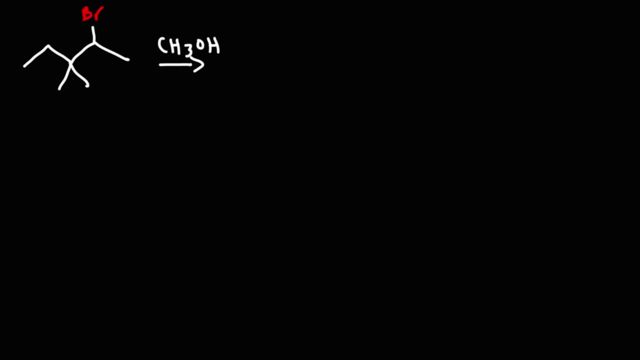 I mean determine the reaction mechanism, the major product, and write out the entire mechanism for this example. So this is going to be an S1 reaction. We have a protic solvent and a secondary alkyl halide. By the way, for those of you who want to know how to determine if you're going to have an S1, S2,, E1, or E2 reaction, 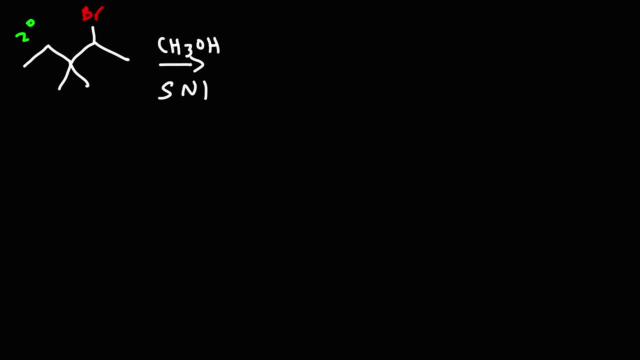 if you're not sure how to figure that out, there's a video that I have on YouTube. If you go to the YouTube search bar and type in S1,, S2, E1, E2- reaction mechanisms- organic chemistry tutor, it's going to show up in the search results. 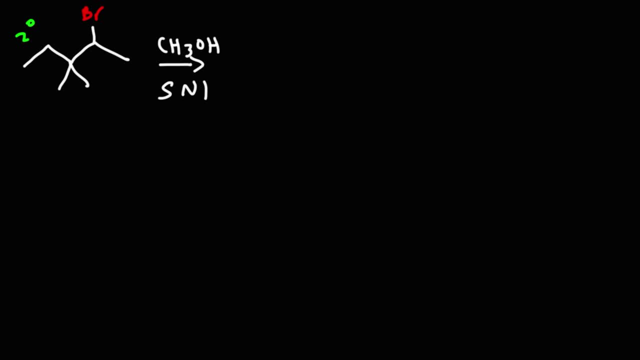 And it's going to give you a table that will help you determine what type of mechanism you're going to have. If you know the substrate- in this case it's the secondary alkyl halide- If you know what kind of solvent you're dealing with and what type of nucleophile you have. 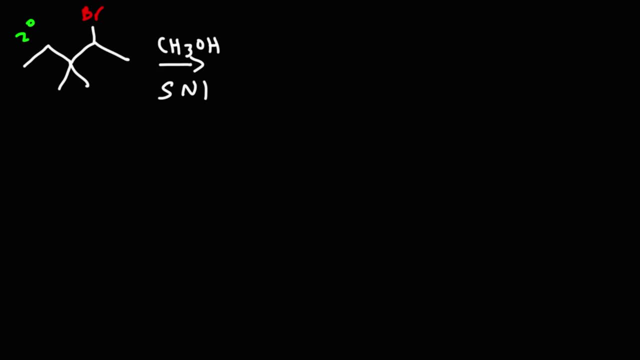 But protic solvents favor S1 reactions over S2 reactions. S2 reactions work better in polar aprotic solvents. Now, in this example, because we have an S1 reaction, the leaving group is going to leave, And so we're going to get a secondary carbocation. 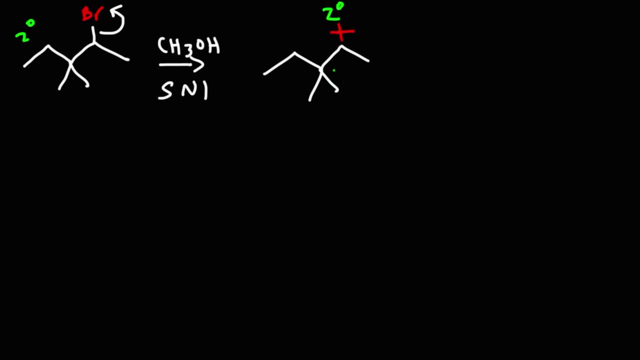 Now this secondary carbocation is adjacent to a quaternary, So in this example we are going to get a methyl shift. This methyl group is going to glide to this carbocation, And so the entire carbon structure of this molecule is going to change. So here's the new methyl group, And this carbon lost the bond. It lost the methyl group, So it's going to have the positive charge. So what we now have is a tertiary carbocation. Tertiary carbocations are more stable than secondary carbocations due to hyperconjugation and the inductive effect. 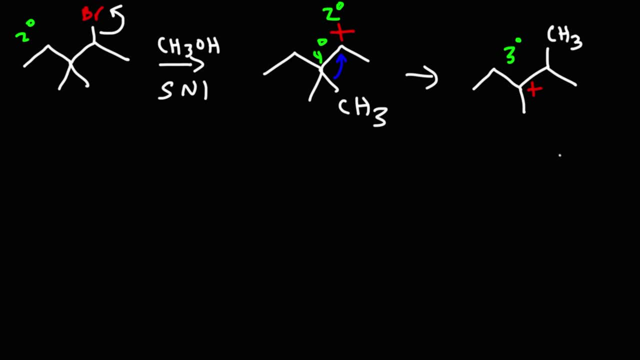 So, now that we have this, what's going to happen? What's our next step? Once we've completed all possible rearrangements, the next thing we can do is combine the carbocation with the nucleophile. So in this case, the solvent is a nucleophile, which means that this reaction is also a solvolysis reaction. 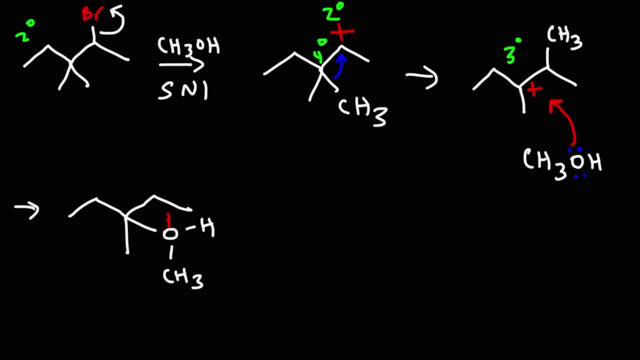 And we're going to get this Now. whenever hydrogen is attached to a positively charged oxygen atom, that hydrogen is highly acidic, So methanol- it's going to behave as a weak base and it's going to abstract a proton. 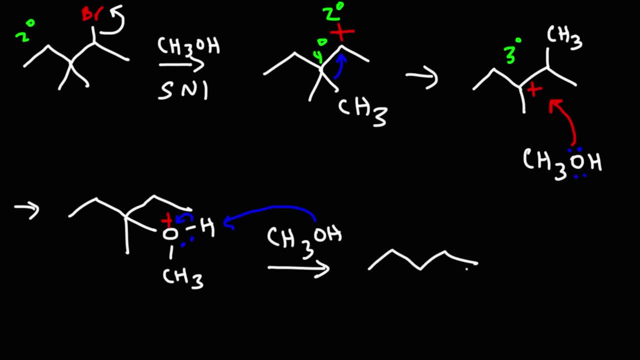 And I forgot this methyl group. So the final result is that we're going to get an ether as the major product instead of an alcohol. So whenever you use water as a nucleophile and if you react to it with an alkyl halide water is going to give you an alcohol. 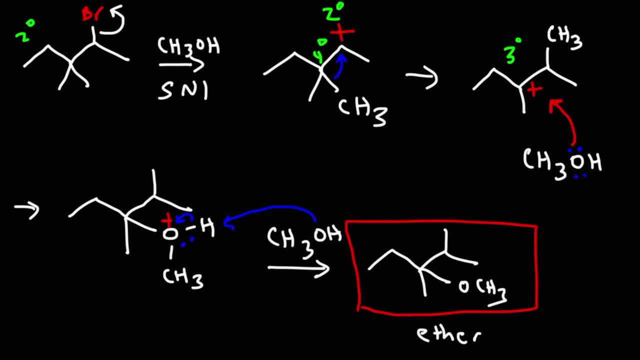 But if you use an alcohol, you're going to get an ether. So that's it for this video. So remember, if you have a secondary carbocation adjacent to a tertiary carbon, you're going to get a hydride shift. 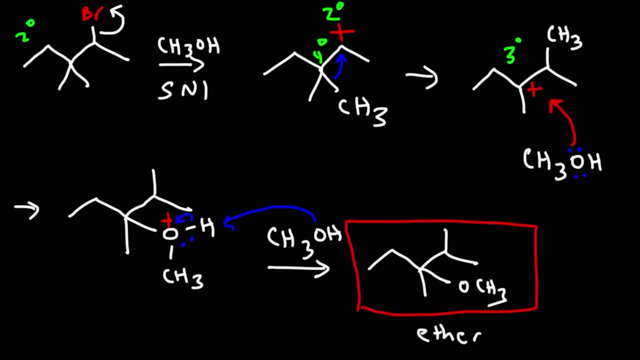 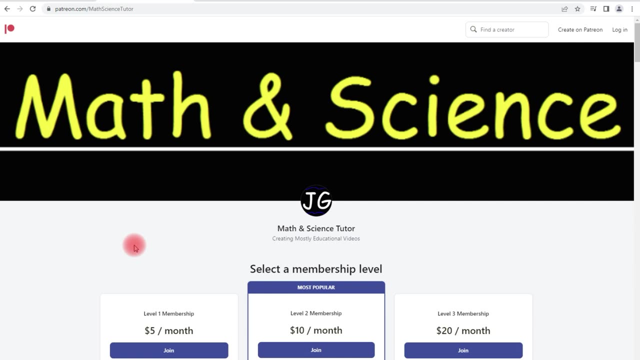 And if you have a secondary carbocation adjacent to a quaternary carbon, you're going to get a methyl shift. Now, the next type of carbocation rearrangement that you need to be familiar with is the ring expansion. Now, for those of you who are interested in this, I'm going to show you a few examples. 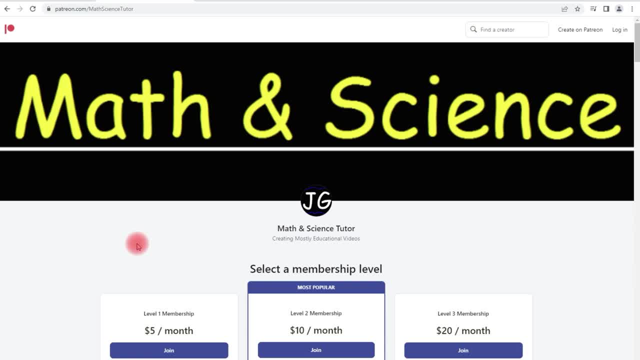 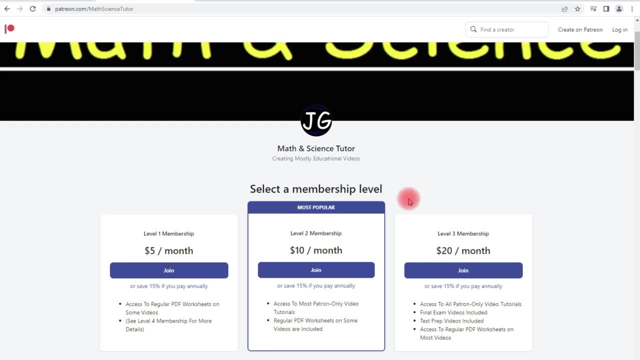 For those of you who are interested in downloading that practice test, here's how you can do it. So if you go to patreoncom, slash math science tutor, it'll take you to my Patreon membership page. Now to get this particular worksheet, you need the level 4 membership. 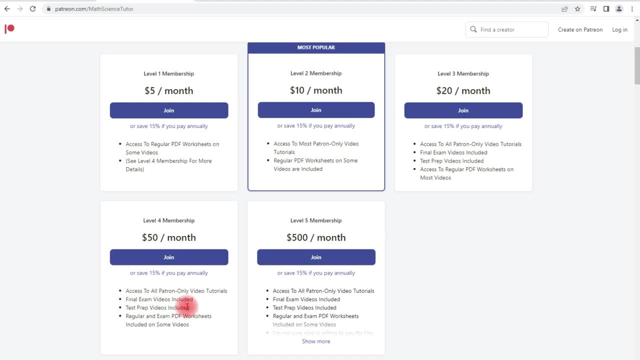 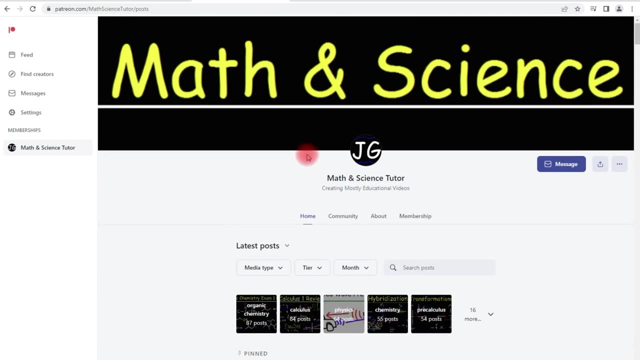 This is where I have my worksheets for final exams and practice tests. Once you sign in, you'll see something that looks like this, And if you go to organic chemistry posts, you're going to get access to the extended versions of my organic chemistry videos.